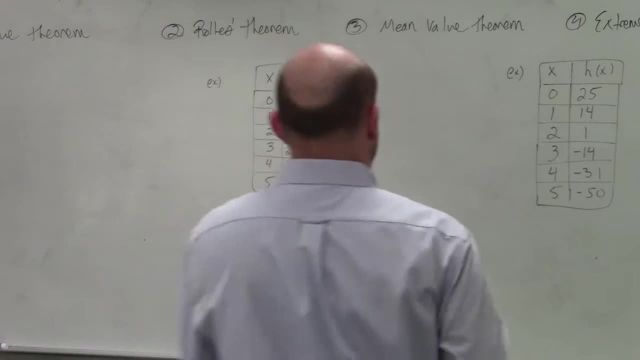 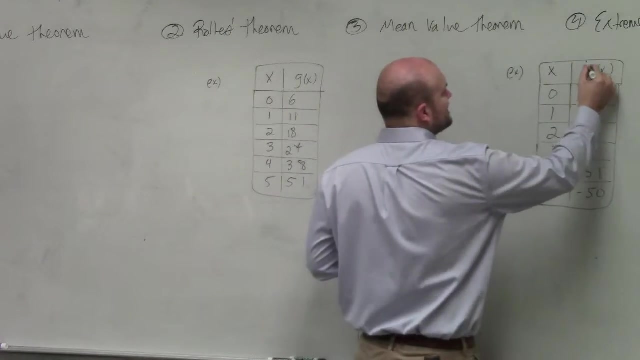 Okay so, and these three examples. I just want to kind of cover this real quick, as one thing that we'll be looking at is- let's just call this one f of x here is identifying if it is increasing or decreasing at an increasing-decreasing rate. 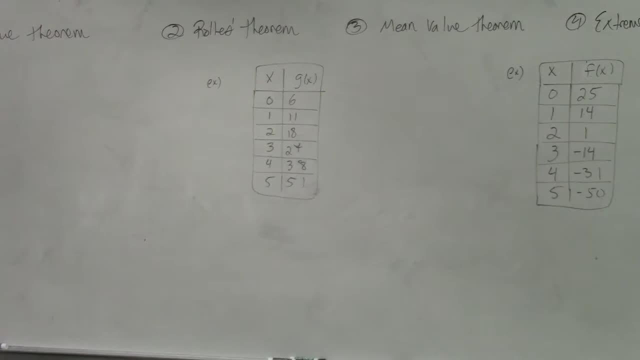 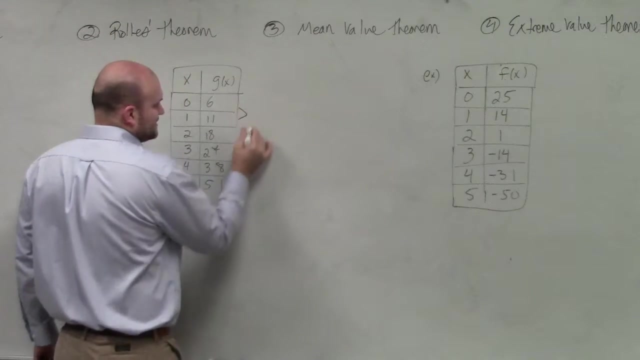 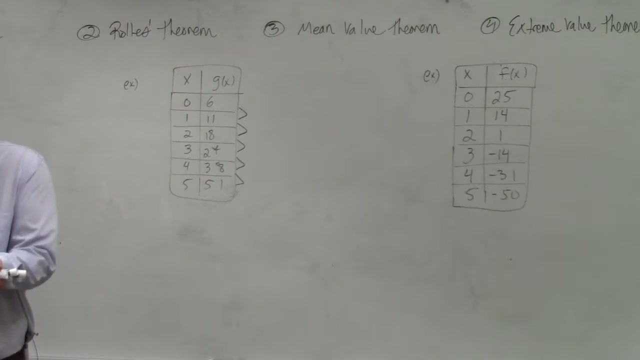 So what I explained last class period, or a couple things that I showed Kevin, last class period- was basically when we're looking at identifying on the function as far as it increasing. we're basically just looking at the first derivative, which would basically be the change within our g of x values, which is the same thing, guys, as like finding our slope right. 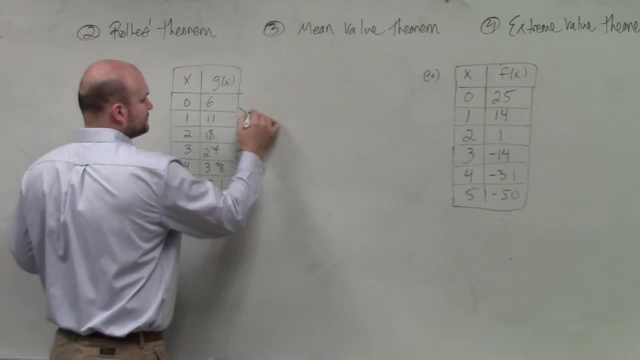 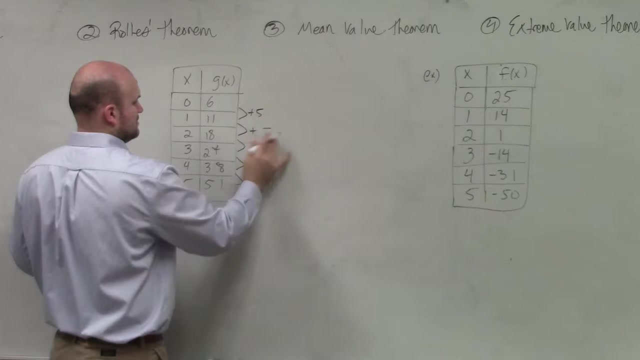 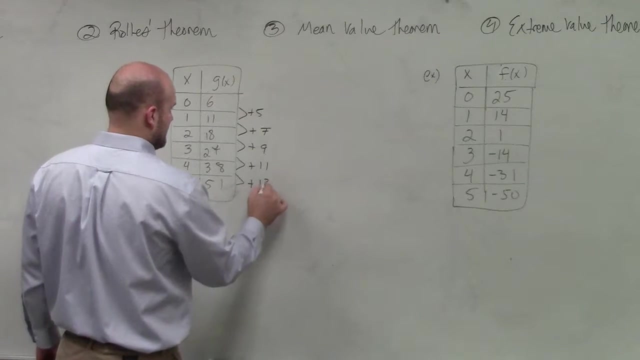 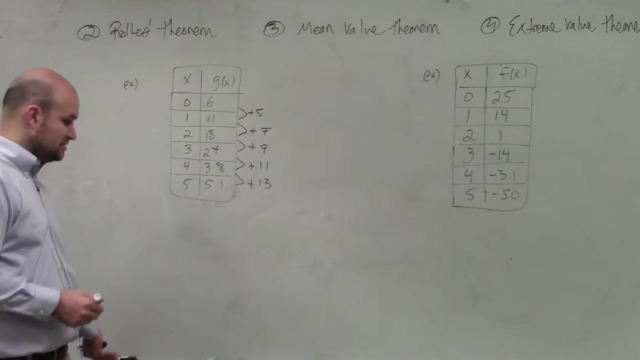 And that's what the rate change is. So you can see, here I'm going plus 5,, plus- oh, I'm sorry, plus 5, plus 7, plus 9,, plus 11, plus 13.. Do you guys agree with me? Right? Then on the next set of changes, you guys can see that again I am increasing once more. 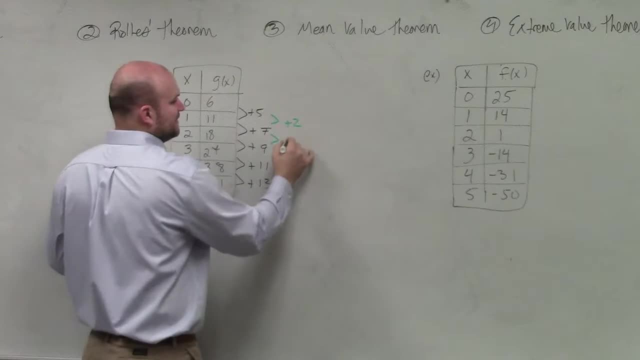 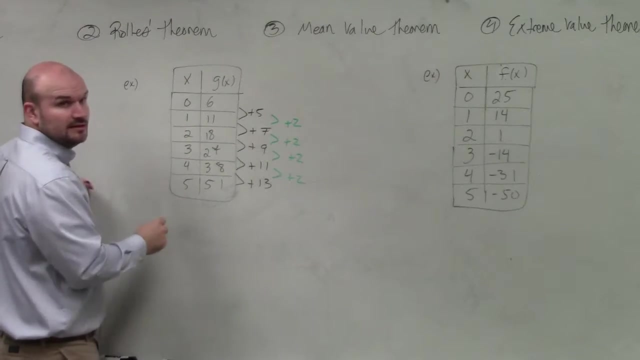 So that the green is going to represent the second derivative. Would you guys agree with me? So what I can say here, Andrew, is: g- a prime of x is greater than 0, and h- prime of x is greater than 0.. 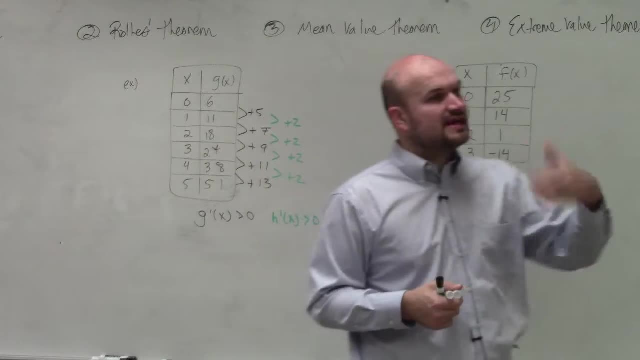 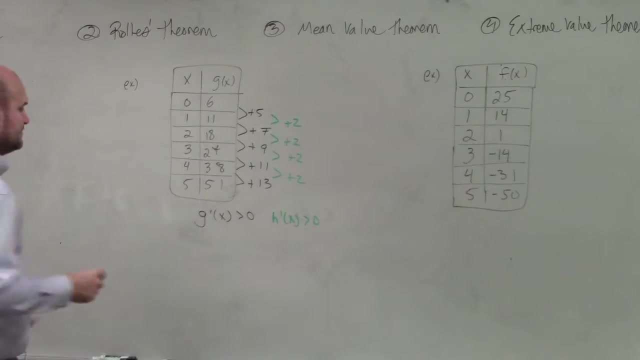 So the main important thing I want you to say is, since the first and second derivative is increasing, what we can say is: the graph is increasing at an increasing rate, It's increasing, It's increasing, It's increasing at an increasing rate. 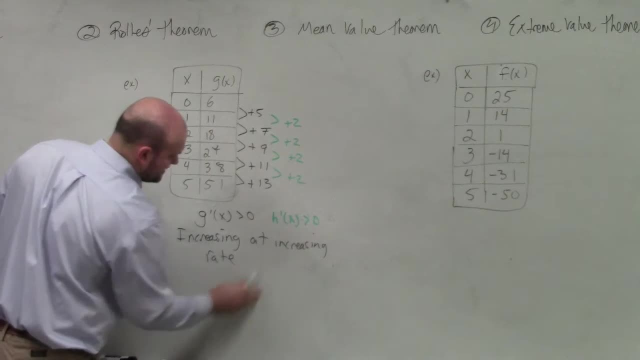 Okay, And if you guys think about like, think about this, think about a concave function, Look at the slopes. Do you guys agree? these slopes are getting bigger, right, And they're getting, and they're increasing at an increasing rate. 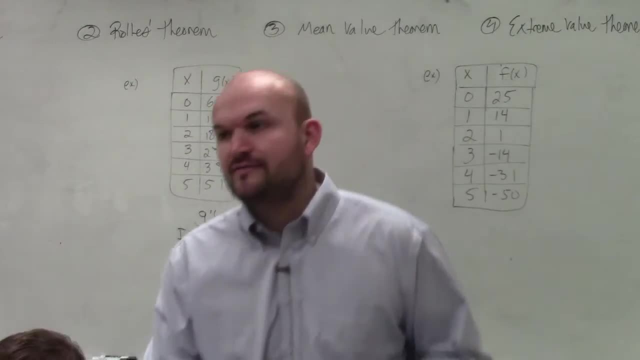 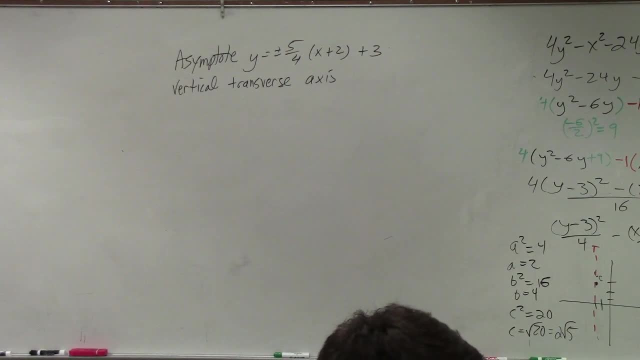 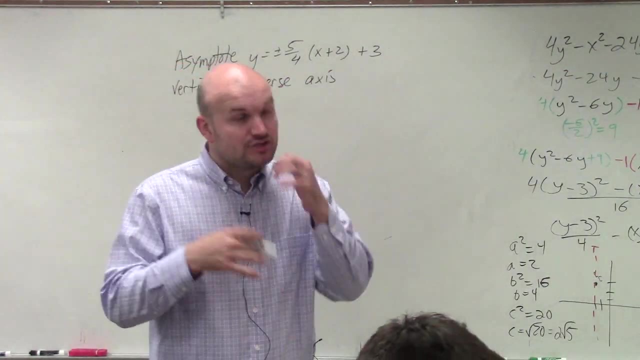 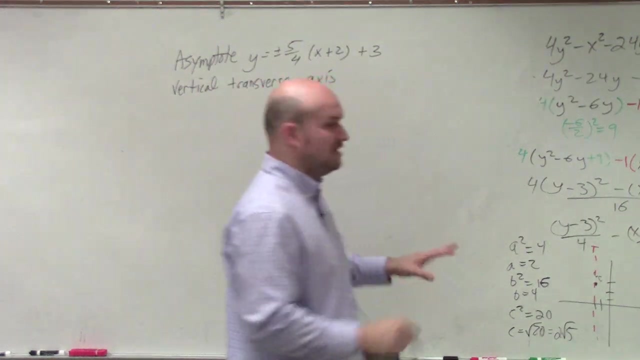 OK, So this problem is actually really not that bad, but it gets a lot of people because the reason is: one, they're talking or two, they don't remember the equation of the asymptotes, Excuse me. So first of all, there's a couple things. 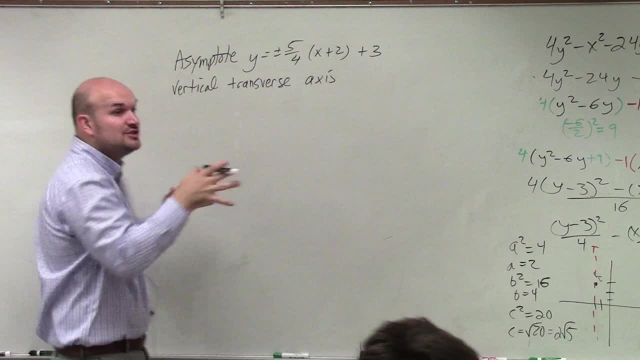 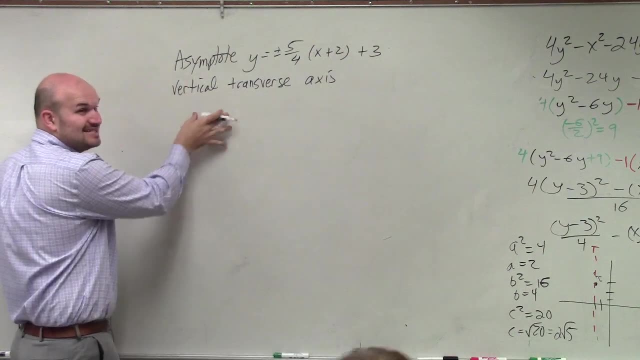 I want you guys to remember, First thing, vertical transverse axis. You guys should know off the bat, if you have a vertical transverse axis, what exactly is the equation of a hyperbola. So remember vertical transverse axis. 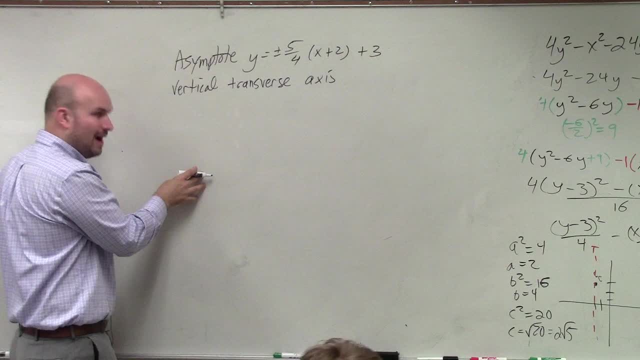 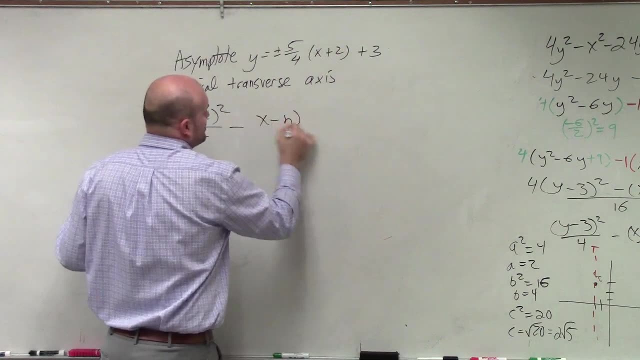 that means my a has to be under my y. So the equation I'm going to use is y minus k, squared over a, squared minus x, minus h squared over b squared, equals 1.. Remember for hyperbola. again we're writing the equation on hyperbola. 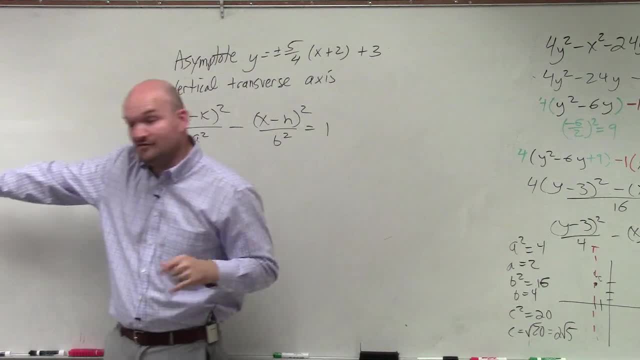 That's what we're practicing today. Hyperbola is always a squared minus b squared. You guys can verify it's over there, But again, those equations aren't going to be on the board when you guys take your test, though, right? 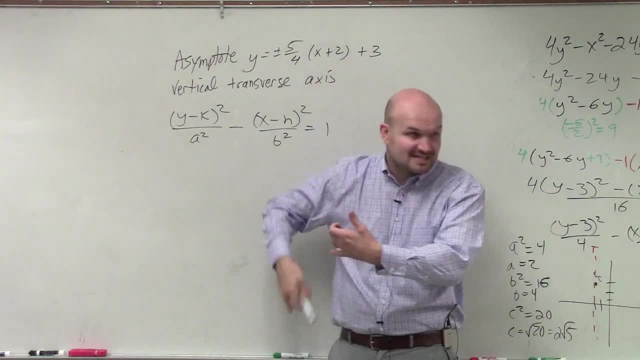 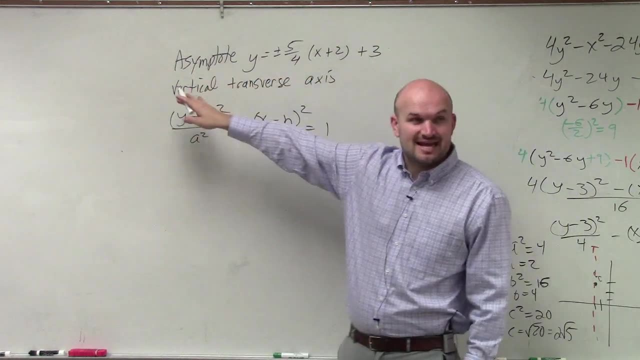 So we've got to make sure we notice. Remember, vertical transverse axis is always going to be a's under That's the y. The next thing that we need to make sure we know is it says it gives us the asymptote. 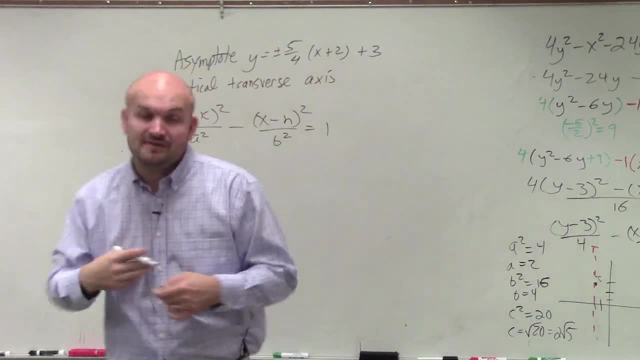 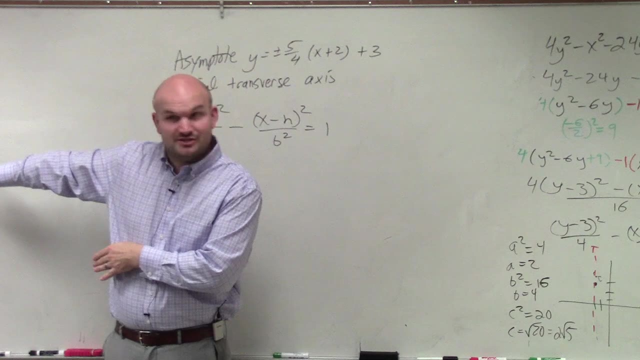 So what does everything mean then? that's on this asymptote. Well, if it's a vertical transverse axis, my equation for my asymptote, I have it memorized. If you don't have it memorized, you're not going to have the availability of it being up.